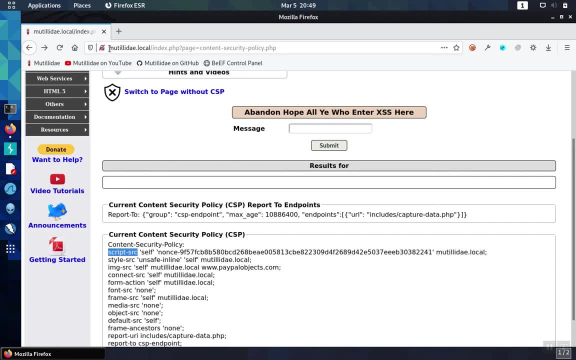 domain. So right now in this application, the domain is matildalocal, So these sources are in reference to that. So we have the self directive which allows us to load scripts from this domain. We've also specified matildalocal here. This example is a little bit redundant. 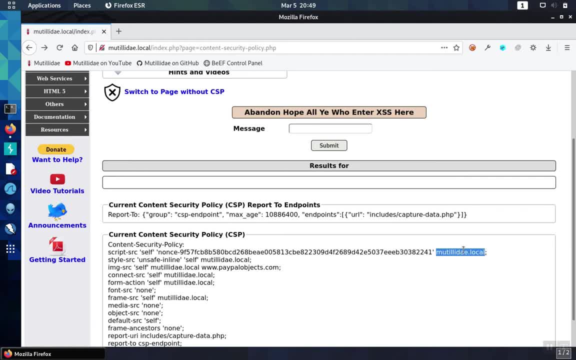 It's the same as saying self, but this could have easily been a partner domain, or it could have even been a subdomain, like API, END OF PARTNER DOMAIN, matildalocal or adminmatildalocal or whatever the case may be, and we also have this nonce. 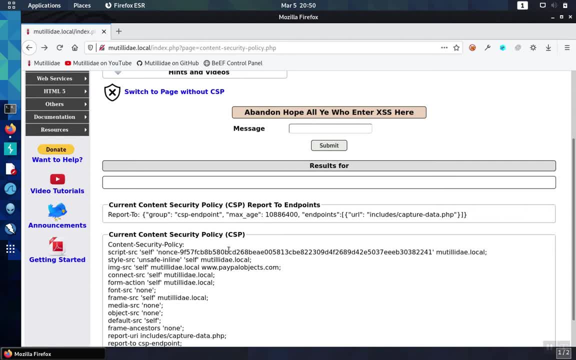 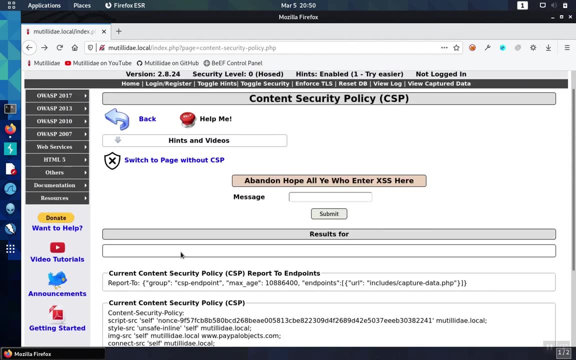 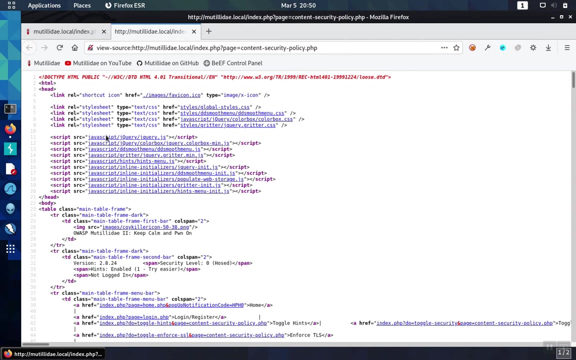 declared as a safe source as well. we'll take a look at the nonce here in a minute. so in this policy we're saying the scripts are allowed to come from essentially us, our domain, or this special case, the nonce. if we look at the javascript behind this page, we'll see that the javascript has intentionally 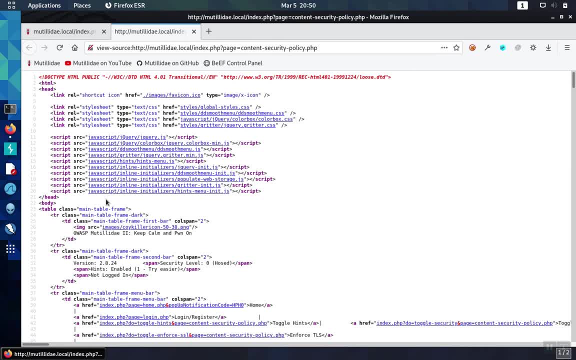 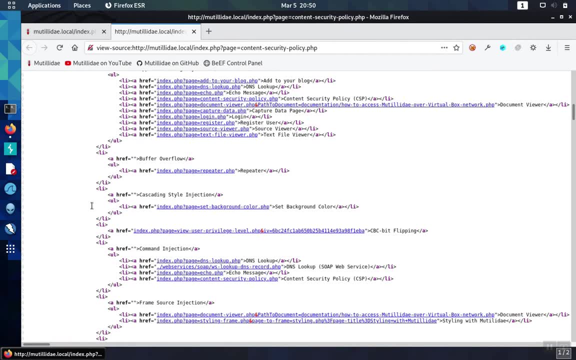 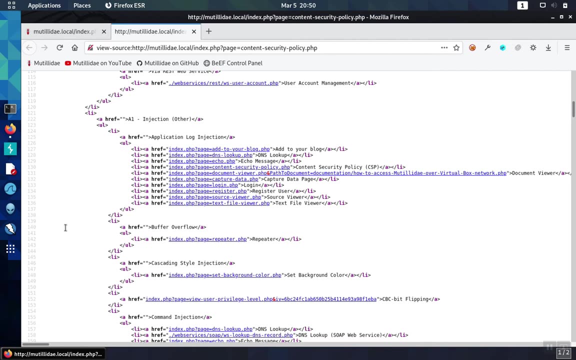 been moved off into js files to be included. in other words, we've removed the javascript from this page and we've done that quite intentionally with because, in order for the browser to enforce content security policy, it has to know when javascript has been injected into the javascript. 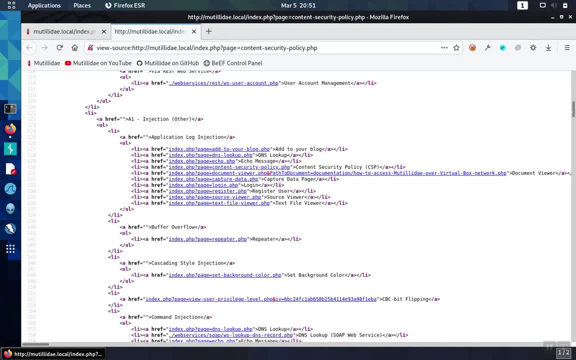 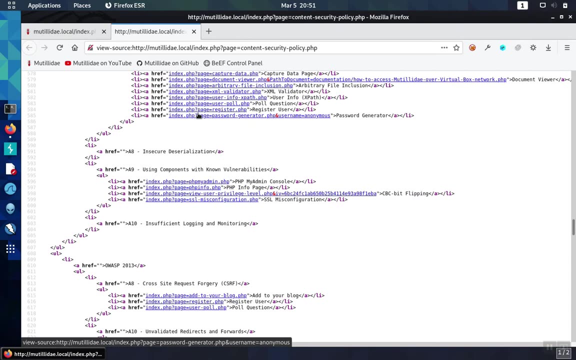 document, and if we are putting scripts in line ourselves, then the browser is not going to be able to baseline the document. now let's take a look at an exception case. so there was one piece of javascript that wasn't removed from this page, down here near the bottom. 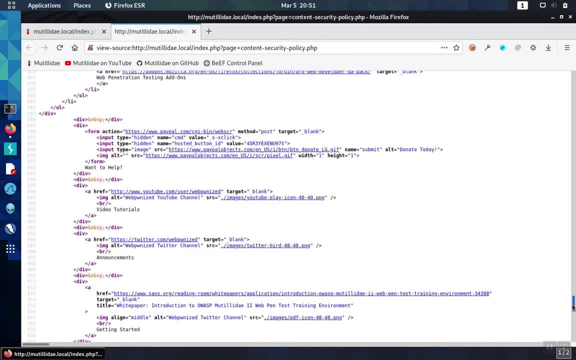 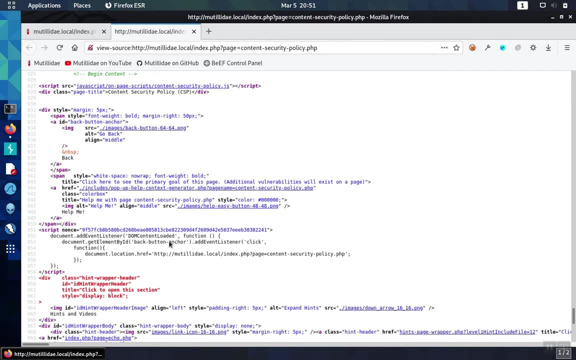 and what this script does is. it actually loads some of the content, creating an event listener for the back button anchor, and whenever this is clicked, then this javascript documentlocationhref fires off and redirects the user. because this javascript wasn't removed from the page, it has to be tagged so that the 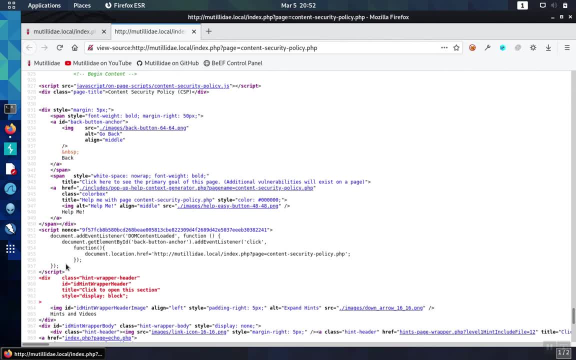 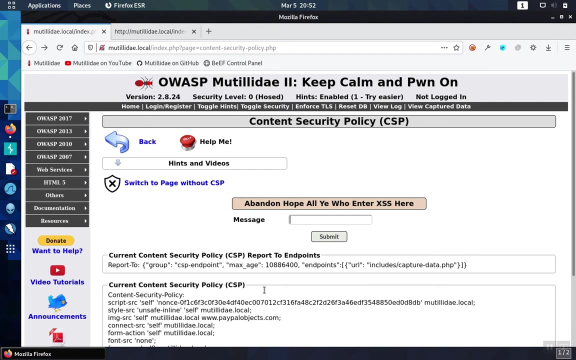 browser knows that this particular inline script isn't originating from an untrusted source, but it's actually coming from the developer. in this case, the nonce was used, so the application will create a cryptographically secure random number on every request and send it back in the response as part of the content script. 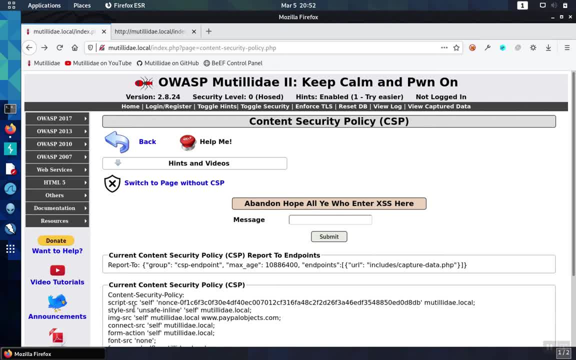 security policy. it'll also put a copy of this number in the nonce attribute of any scripts tags that are going to be included in line. the browser can match the nonce declared in the content security policy against the one declared in the script tag and make sure they match. 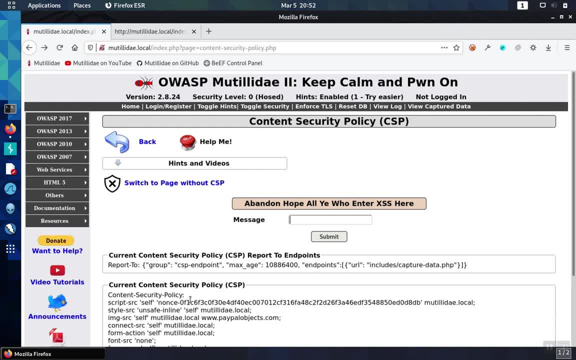 since this random number is never repeated, then there are not going to be collisions. it's not technically impossible for the number to repeat, but that's why we need to use a cryptographically secure random number, because, statistically speaking, a secure random number is not going to repeat. 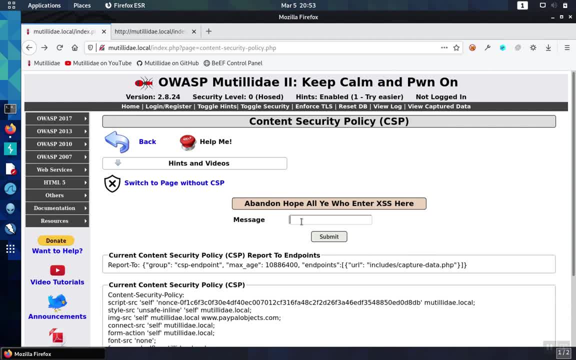 so now the browser knows the safe places that javascript can come from. so what happens if javascript comes from somewhere else? for example, what if a cross-site script is injected into the page? so let's say we had a script that tried to read the contents of the cookies on the page. 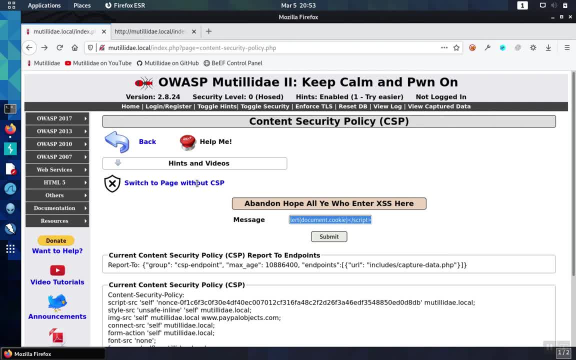 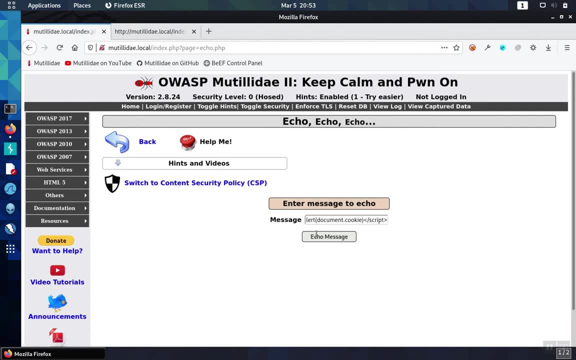 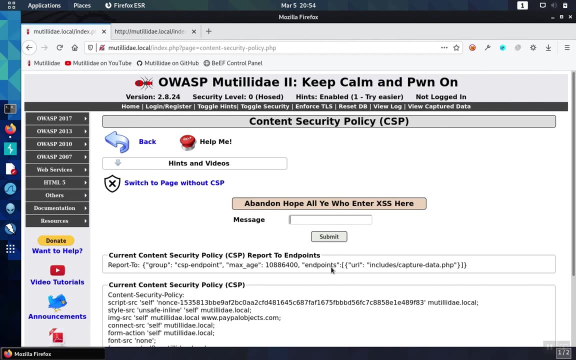 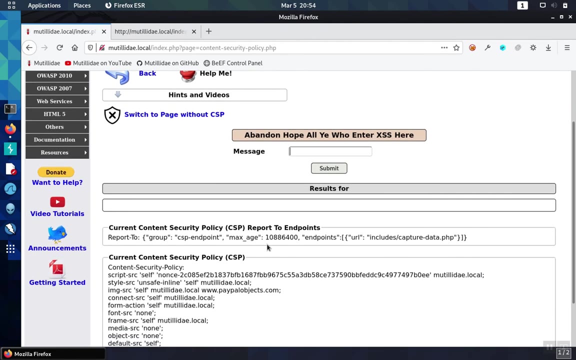 so we write our script and let's go to a page that doesn't have content security policy protection, just to make sure that the injection works. so the script works. we go back to the page protected by content security policy, we inject it, And at this time the browser knew that the script was not coming from one of the sources that's allowed by content security policy, so it automatically blocked the script. 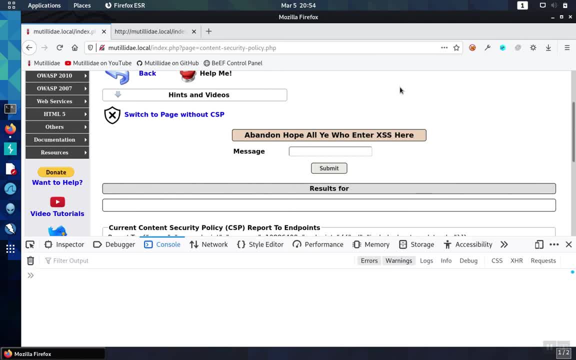 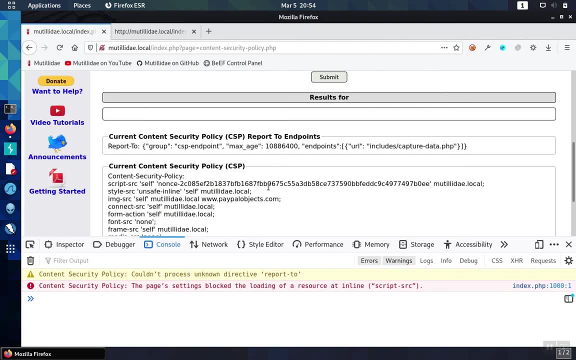 You can see a message indicating such if you look in the web console. The other blocking content security policy directives work in a very similar way: Style source, image source and so on. You declare a list of domains, including the current domain, where content is allowed to originate from. 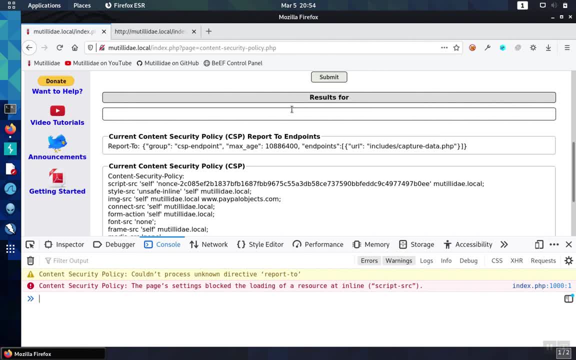 If that type of content shows up from anywhere else, including inline injections, cross-site scripts and other domains, the browser will block that resource from loading.